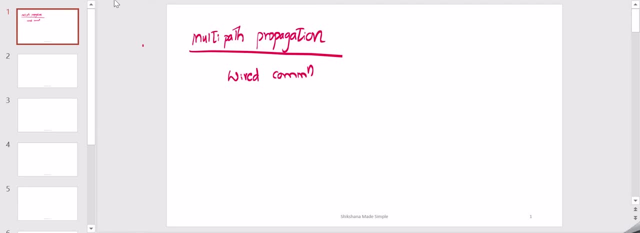 there on. I will pick on the concepts related to multipath propagation. all right, so we'll see the difference first. so in what we invite, communication, as we know, if there is a transmitter and the receiver, between transmitter and the receiver, we will have a dedicated cable right. so the signal 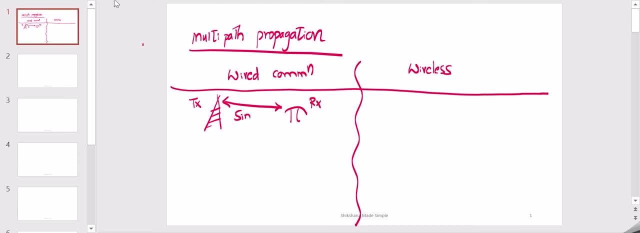 via this cable in only one path, that is, a single path. all the signal will contain within the cable. so what happens, since there is only one path available, would be the receiver. receiver looks very simple, receiver is simple, okay. so so since there is only you know, since there is a cable running between transmitter and the 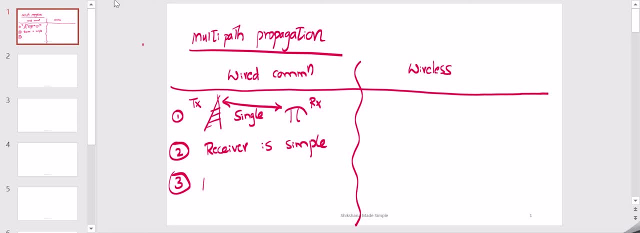 receiver. and how about the infrastructure? infrastructure is very huge, right, you need a huge infrastructure, so we. so this makes the system very costly and lot of maintenance is required. so now, now, let us start with multipath propagation. so let us start with multipath propagation. so let's come to wireless communication systems. so in this, the signal is transmitted from the 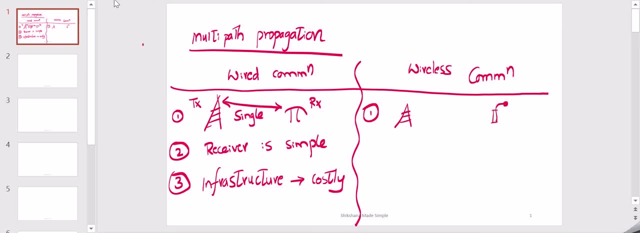 transmitter to the receiver. over the year, the signal will travel in multiple directions and it will reach the receiver cut, so here we will have multipath. so since the signal reach that the receiver have a multiple components, how do we have to process it? we need to take care or we need to ensure that the signal, the signals, are received. 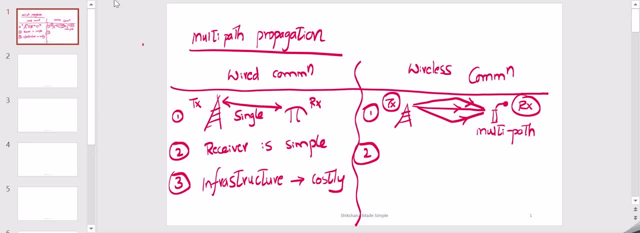 at receiver are processed properly so that it will help for further, further processing. so if we don't process it properly, there may be a chance that we might lose the signal. okay, so because of that reason- uh, you know- the receiver becomes very complex, there is more processing involved and 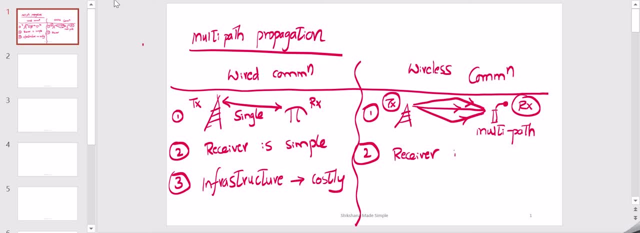 and hence we need a complex receivers. of course, infrastructure wise, compared to wide communication, it is pretty much uh simple and it could lead to less cost. but there are many other challenges related to uh, related to wireless communication. so if you can overcome those uh challenges, okay, by processing the signal. 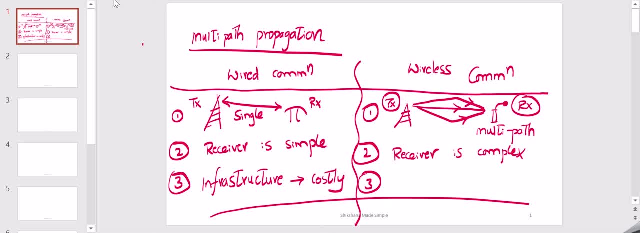 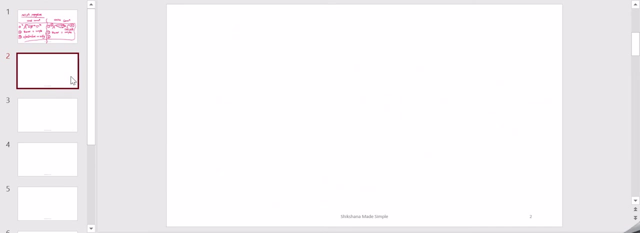 very efficiently, then we can get much, much bigger benefit in case of wireless communication. so these things we will see in the upcoming videos, but, uh, for now, uh, we will focus on in this video, we will focus on the multi-part thing, okay, so now. now we will see why. why, uh, signal uh? 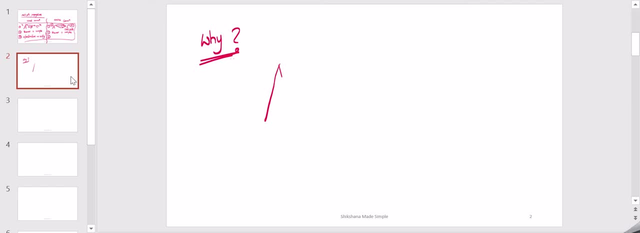 traveled in multiple directions. okay, so there was a transmitter and we had a receiver, so the signal is transmitted over the air and over the year. we have got many phenomenons right, like if we. if you go back to your physics concepts, there are many concepts which will apply over here. 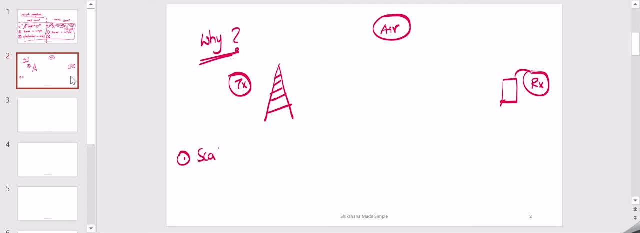 the first one is scattering. so in case of scattering um the signal, uh, when, when the signal eats, uh, a particle, okay, let's say, this is a particle, this is, let's say, the signal is transmitted and it hit the particle and from that particle the signal would travel, uh, in multiple directions. so this scattering will happen when your signal. 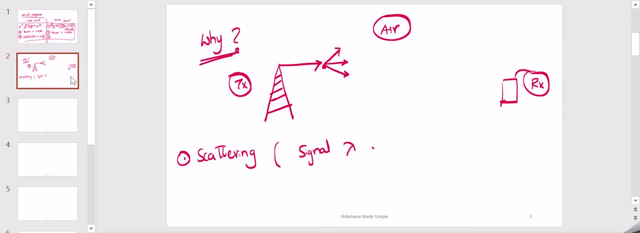 wavelength. so signal wavelength is order of uh, uh, uh, uh. i mean signal wavelength is approximately same as the size of particle. so so, uh, so what happens? let's say this is the like signal with power p, but after hitting the particle, when the signal scatters, uh, there is some. 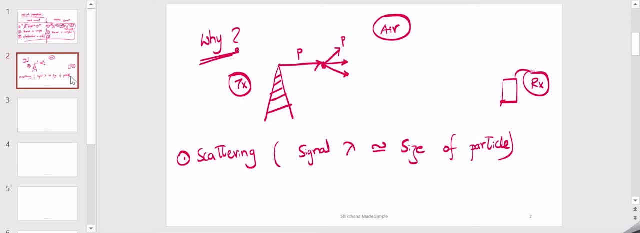 reduction in the power. okay, let's say here, for time being it is uh, p by 3, p by 3, p by 3, so then this signal would continue and it will hit another particle, let's say test, transmitted in multiple directions, and like that it will, it will reach. this is one of the path, part of the. signal which has reached the receiver. this is happening because of scattering, and this is going to be techniques. we will see also. next I'll show something over here and then we will come to a contouring target. and now you know it爵, Mustafa, itfilled, uh, the path. Anyways, this signal has reached the receiver and this one is happening because of scattering. this one has matin. 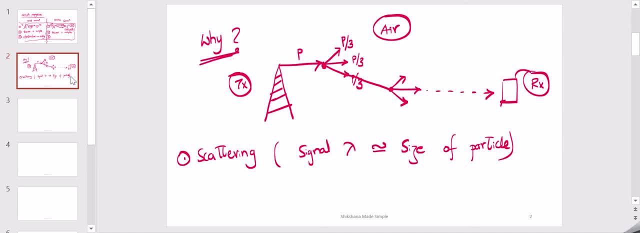 file. that would also help если we want to see that this video will take you where, and later we will talk about the fact that there are six, very, very few directions. so, if you would like to, of scattering, as you can see that as signal travels, there is a reduction in the power. 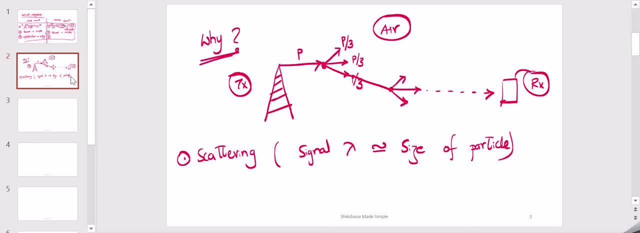 right due to scattering, and that that relation we can bring it with the path loss as well. so, but for now, one of the component is one of the factors which is resulting in multiple directions is the scattering. okay, let's say this is path number one now, here in scattering, i want to mention one more thing, that is: 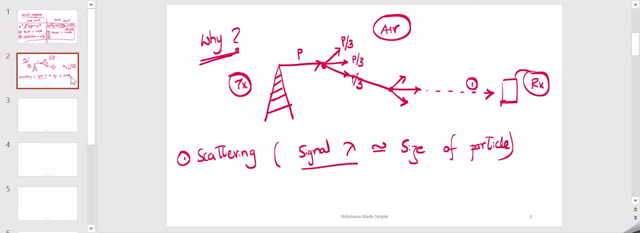 i was mentioning that signal wavelength should be having you know the size, which is equivalent to the size of the particle. now, now let us say: usually what is the size of the particle? it's very, very small, right, very small. so very small means it could be in, in, in, in centimeters, or it would be in millimeters. 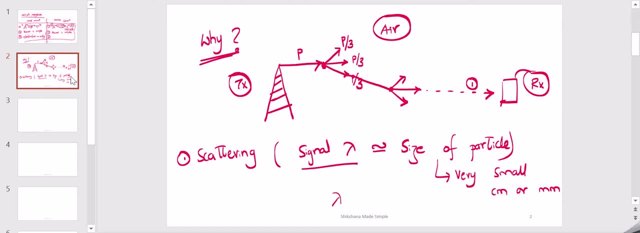 so if your wavelength is very high then then then what happens to scattering? wavelength is very high, scattering will be less. but if wavelength is very small, then your scattering is very high. so when you move from actually centimeter waves to millimeter wave, you see that the scattering is very high. all right, 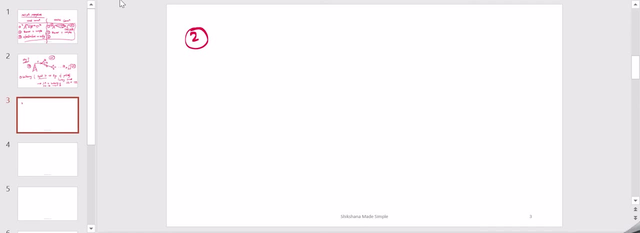 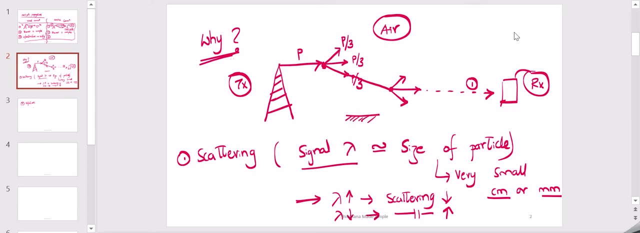 the second concept which i want to talk over here is the reflection, so between the transmitter and the receiver. okay, let me go back to the same picture. let's say you encounter one kind of a reflector over here. so let's say, signal transmitted in this direction and we did the surface and it reflected back and reached. 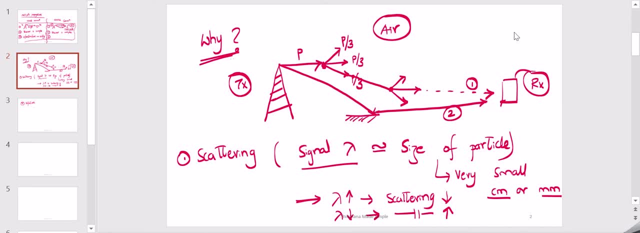 the receiver. so here also there will be some loss of power. there could be some absorption, and then there is a reflector- because reflectors need not be a idealistic reflector- where whatever signal uh with power p is coming, uh, the same power will be reflected. it will be usually like if the power p is hitting the surface, then it would be a p dash. 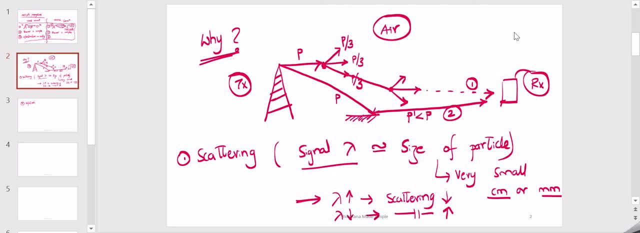 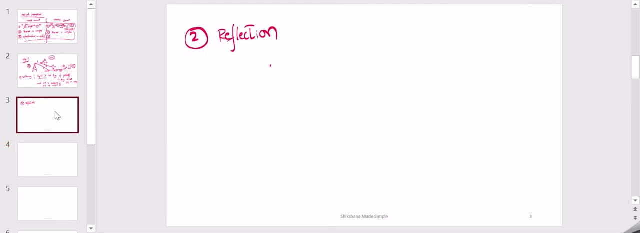 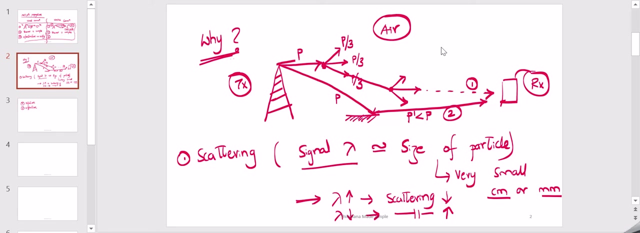 less than p, okay, some absorption will be there and hence we will see a little bit less power over, less power at the receiver. so what about the third concept, which is the diffraction? so in case of diffraction, let's say: uh, the signal has transmitted from this direction and it is meeting an obstacle which is sharp obstacle, so it hits the obstacle. 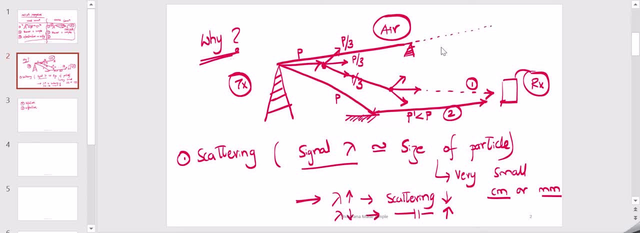 and the. actually, the signal is supposed to travel in this way, but because of obstacle, you you can see that the signal has been diffracted and it has reached the receiver in this direction. so this is another phenomena where, uh, you know, you will see that there could be a multiple. 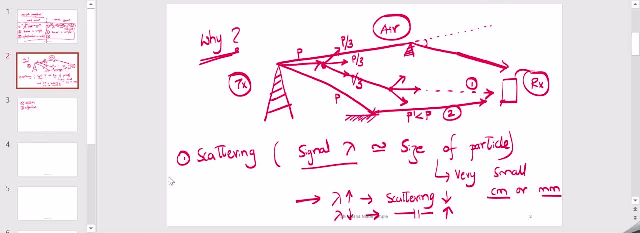 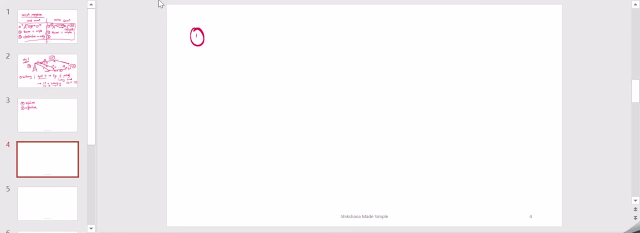 uh, component of the signal. all right, we have seen the three uh uh different phenomena because of which we can have multipath components, so I want to talk about a couple of basic concepts in order to you know, model the signal which is received at the receiver. okay, so the first basic concept is the path loss. so, path loss. 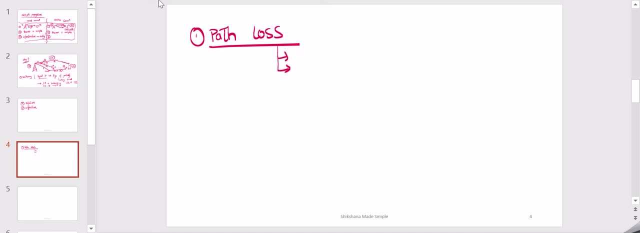 as I was telling, in scattering also we will do some. in reflection, in diffraction also we will. in all these cases we will lose some amount of power. okay, but these reduction in the formula has been modeled, has been modeled and we see that if we go through the equation. 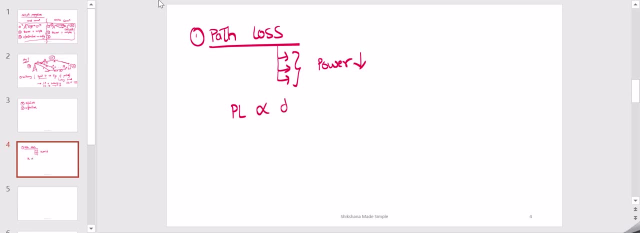 of path loss, you will see that the path loss is directly related to D by lambda. okay, so which means if the signal travels more distance, there could be more scattering, and because of which, there is a more path loss. or let us see if we have the signal with the wavelength. 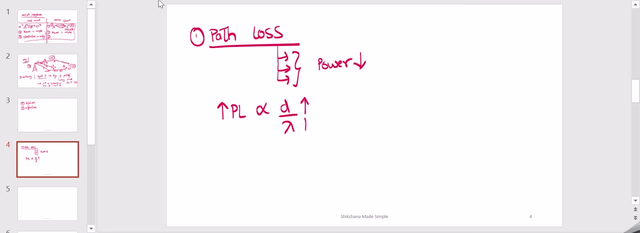 with certain wavelength. so let us say, if wavelength is going too low, maybe from meters to centimeters to millimeters, then we will see that the path loss is going to be more or less like this: path loss is very high. or in other words, we, if we talk about frequency, if we are going 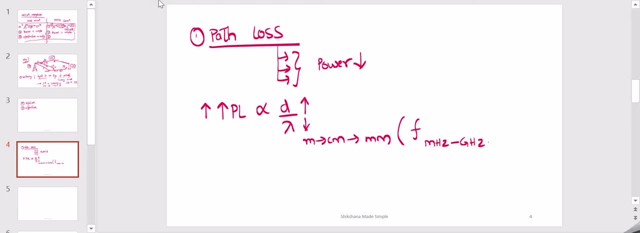 from just to megahertz to gigahertz, to, you know, greater than 30 gigahertz of like that, then then we will see that there is a. so here the frequency is increasing. your path loss will increase, all right. so if we take the equation, we will see, I mean, how this is incorporated in the equation. but 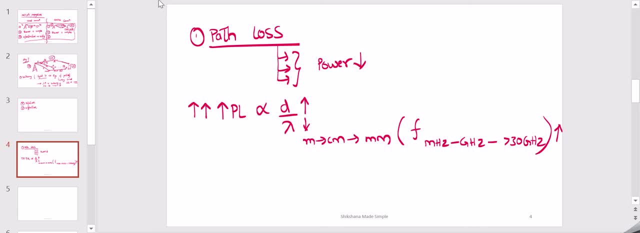 right now. you got the concept that if the signal travels a longer distance, you will see the path loss. okay, the second thing which I want to explain is the delay because between the transmitter and the receiver, if the signal is increasing, and this is very much related to the way it is happening. if you smell this, ощущ happy. 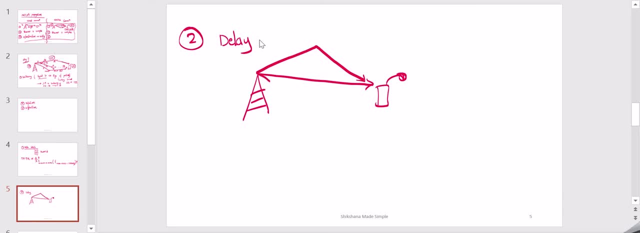 you know, not only will it be very late condition, but the the result will be very low. it will be applied if we are just fix um aithmetic variation is just is happening here in, or something like that, because the signal is very muchぐll. shows you, Anthony, raise finger. 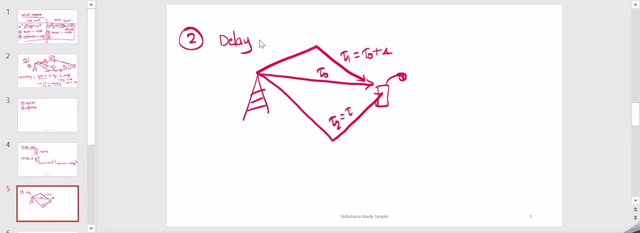 as you go further, you can see we are here for tantrumU slightly to deeply, if we should be lost. okay, so there is a. there is a different delay, which is which should be applied to each of the multipath components. so then, what do we say about the signal? 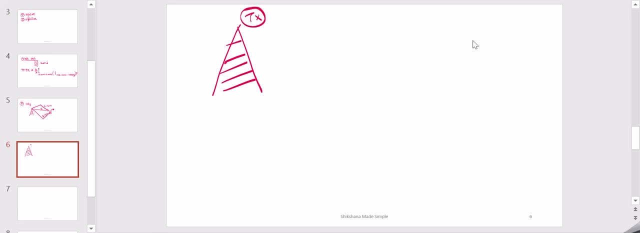 received at the receiver. so let's say there is one component which is a line upside component, and now let us say there is one more component and finally i will put three dots. and then there is another last component. let's say total. there is a, l is equal to a number of multipaths. 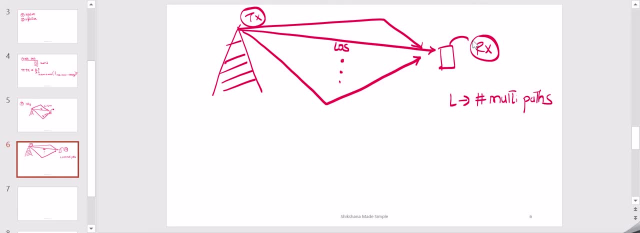 so then then we can say that y of t, this is x of t which is transmitted. so it is the same signal which is traveling in all these uh directions, but, uh, these signals will underway different kind of channel effects and it will reach the receiver. so at the receiver we are supposed to get the same signal, x in the line of sight. let's say this is: 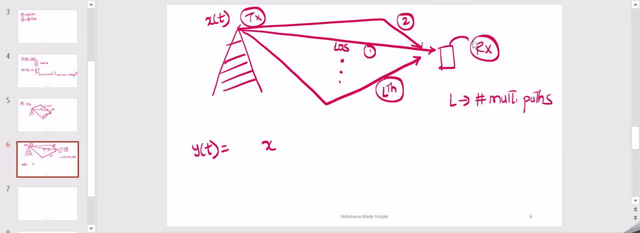 first part, second part and this is lth part. so first part: uh, let's say x1 of t plus x2 of t plus xl of t. so what about x1, x1? let's say: uh, it has, it has undergone some attenuation and it is a naught. a naught corresponds to, i would say, ai corresponds to amplitude. 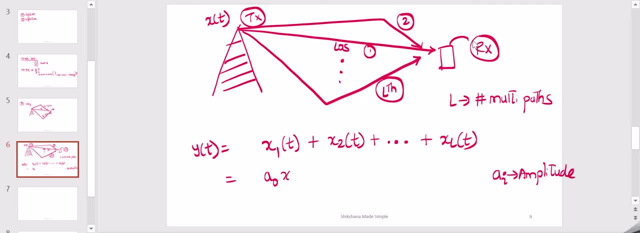 amplitude of the signal. so now this is x of t minus 12 zero. so these are all delays, now plus x2, which is uh, so a2 actually. uh, oh, one second, so, oh, so, okay, let me write it and delay. so this is so here the what is the condition? the condition is: 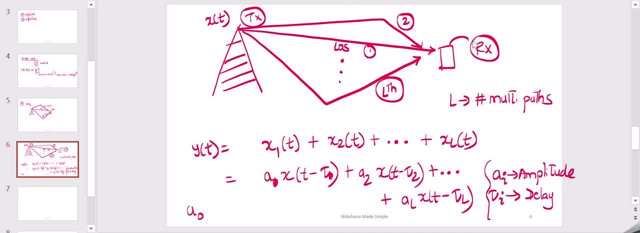 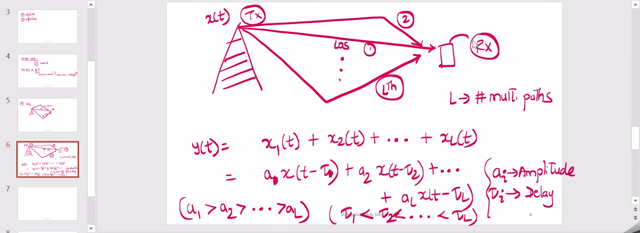 so your a1 actually amplitude will be greater than a2 and it will be greater than al right and in terms of delay as well. what is the condition? so your tau 1, actually this delay will be less than tau 2 and tau l. so i hope this is clear. 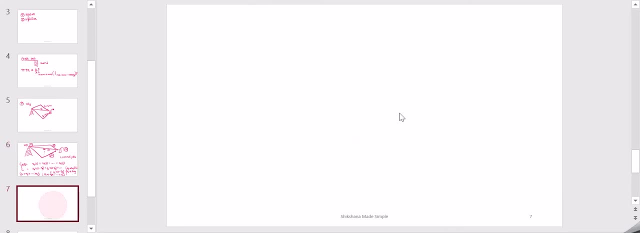 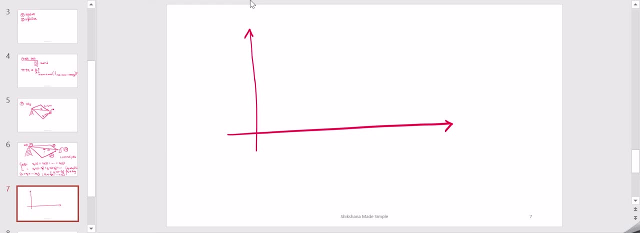 i want to just show in terms of, i want to just show in terms of some, some, some um, um, um, diagram, diagram, diagram. so this is, let's say, time, this is let's so, this is, let's say time, this is let's so, this is, let's say time, this is, let's say, amplitude. 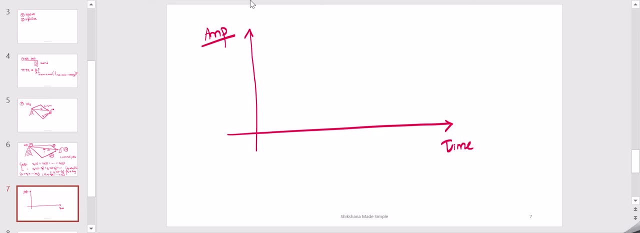 say amplitude, say amplitude, okay. so this is, let's say okay, so this is, let's say okay. so this is, let's say the reference point, the reference point, the reference point, so the first component received at uh, so the first component received at uh, so the first component received at uh, which is: 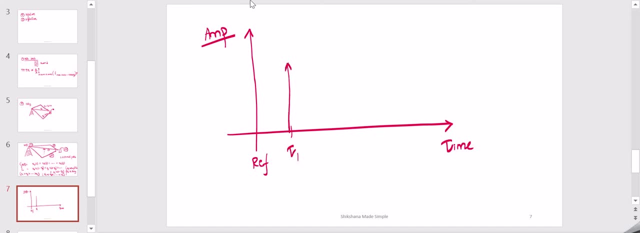 which is, which is tau 1 right at tau 1. if you see it, tau 1 right at tau 1. if you see it, tau 1 right at tau 1. if you see it, there is a signal with the greater, there is a signal with the greater. 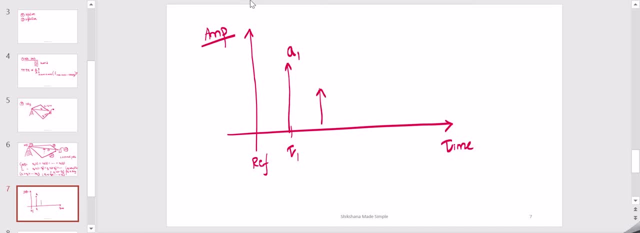 there is a signal with the greater amplitude a1, amplitude a1, amplitude a1, then at tau 2, then at tau 2, then at tau 2, so tau 2 is so tau 2 is, so tau 2 is late. and here, if you see, 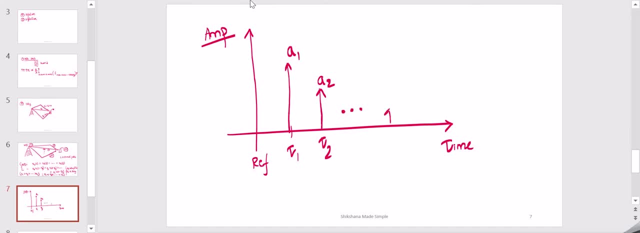 late. and here, if you see late, and here, if you see this is a2, this is a2, this is a2, then then, then, finally, we will have al at. finally, we will have al at. finally, we will have al at. if you see, if you see, 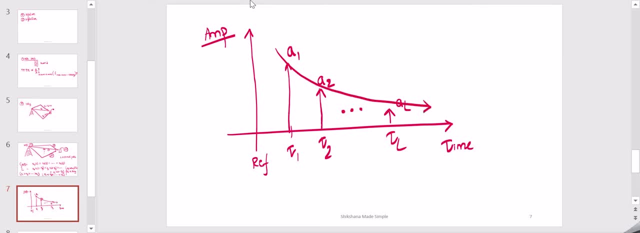 if you see, you know the signal amplitude is, you know the signal amplitude is, you know the signal amplitude is getting reduced, getting reduced, getting reduced as and when it travels a longer as and when it travels a longer as and when it travels a longer distance and distance and 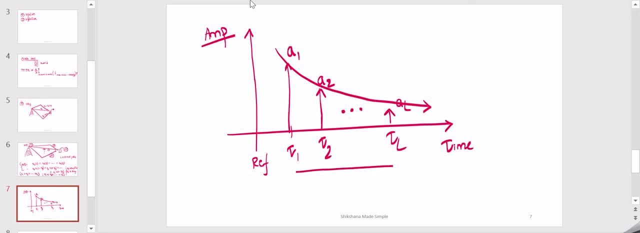 distance and and also like as and when it travels, and also like as and when it travels, and also like as and when it travels- longer distance. you will see that longer distance. you will see that longer distance. you will see that the delay is also. the delay is also. 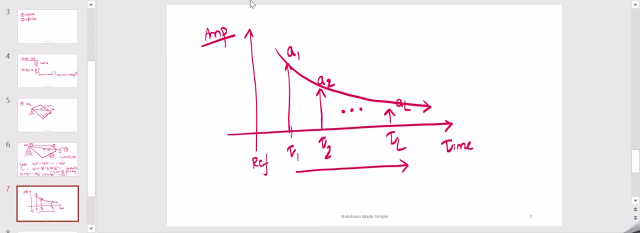 the delay is also increasing, increasing, increasing with this. i want to stop in the with this. i want to stop in the with this. i want to stop in the upcoming video. i will talk about upcoming video. i will talk about upcoming video. i will talk about one of the effects of the multipath. 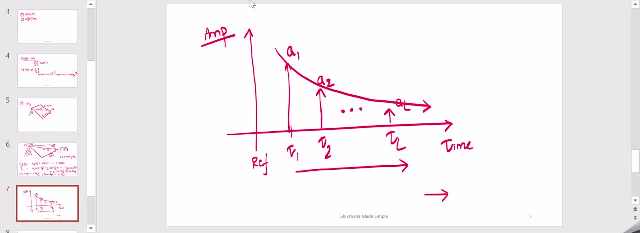 one of the effects of the multipath, one of the effects of the multipath. so multipath will lead to a. so multipath will lead to a, so multipath will lead to a. a important concept in a important concept, in a important concept in wireless communication that is called. 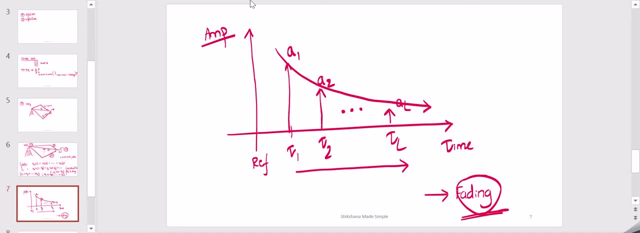 wireless communication. that is called wireless communication. that is called fading, which is a multipath fading. fading, which is a multipath fading, fading, which is a multipath fading. we'll talk about fading in the. we'll talk about fading in the. we'll talk about fading in the upcoming video. 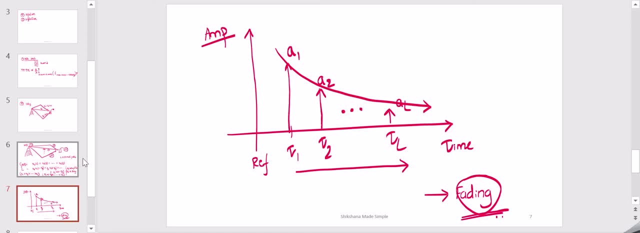 upcoming video. upcoming video. thank you, my dear friends, please do. thank you, my dear friends, please do. thank you, my dear friends, please do subscribe if you like this video. subscribe if you like this video. subscribe if you like this video. and there are many more upcoming videos. and there are many more upcoming videos. 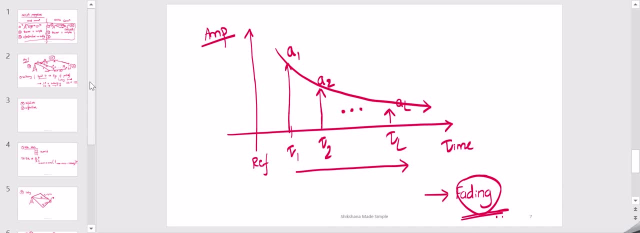 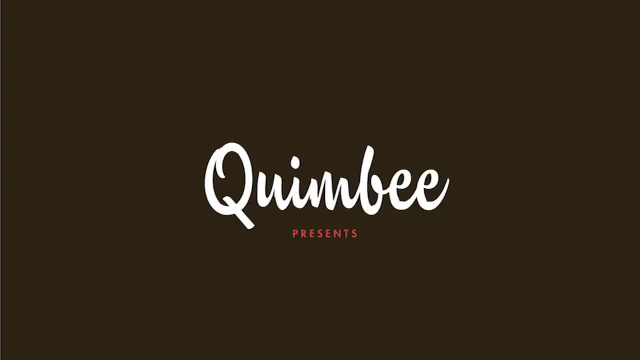 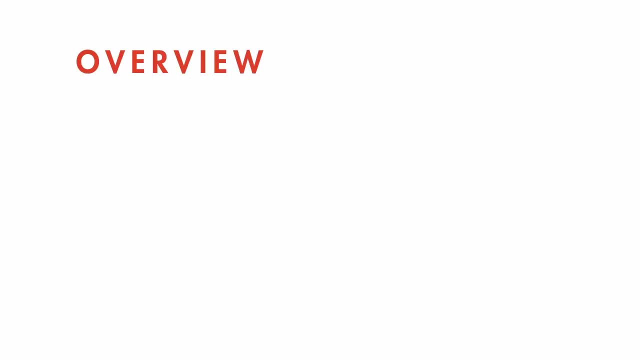 We have discussed the significance of confidentiality in the lawyer-client relationship throughout our tutorials and clips. The model rules as a whole place great value on a lawyer maintaining a client's confidences. Now we'll look at the source of the general rule of confidentiality contained in Model Rule 1.6a. In this clip we'll discuss the significance of confidentiality. 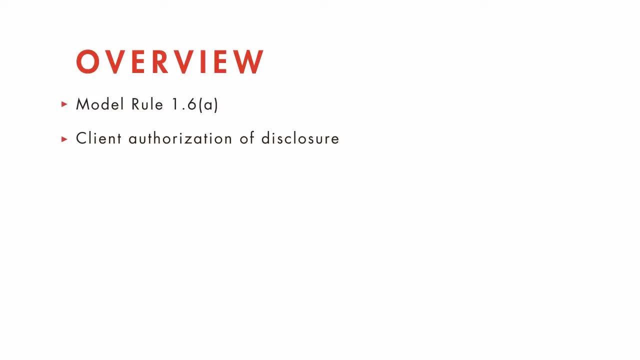 discuss how a client may properly authorize disclosure by giving their informed consent and compare the general rule of confidentiality with the attorney-client privilege and the work-product doctrine that we have just reviewed. Then we'll have a brief summary and a quiz to reinforce what we've learned. 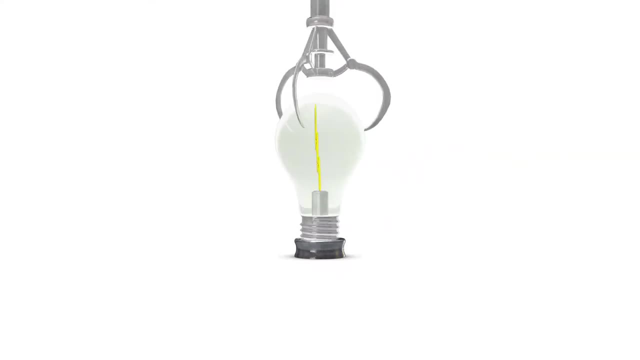 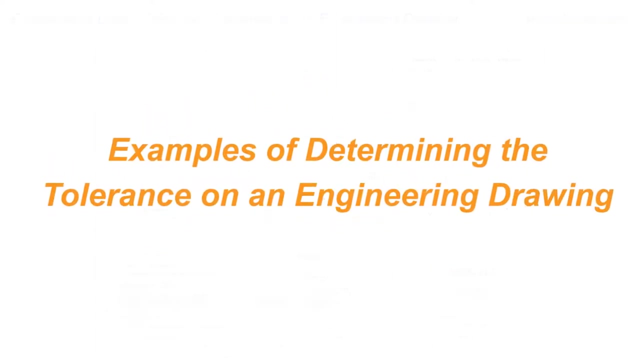 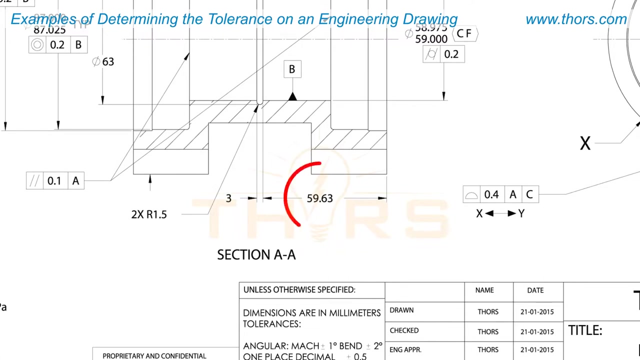 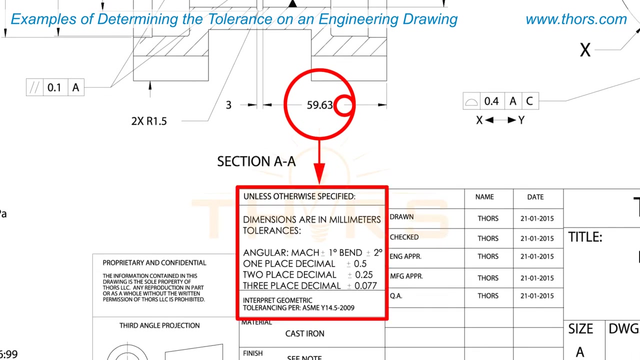 Tolerance information can be located within the drawing itself. If a dimension does not have a tolerance beside it, the tolerance for that dimension will be referenced in the title block. Whether the drawing displays imperial or metric units, the same manner of determining the tolerance.